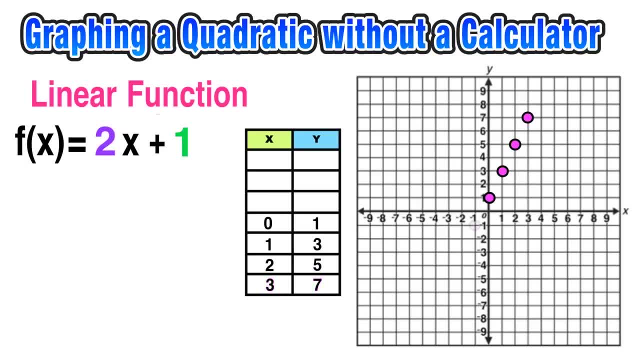 that one more time to get the point 3, 7.. Now I can also go in the opposite direction below the y intercept to find more points, and then I can connect these points by constructing my line, and that was pretty easy. So for a linear function, our starting point is that y intercept. 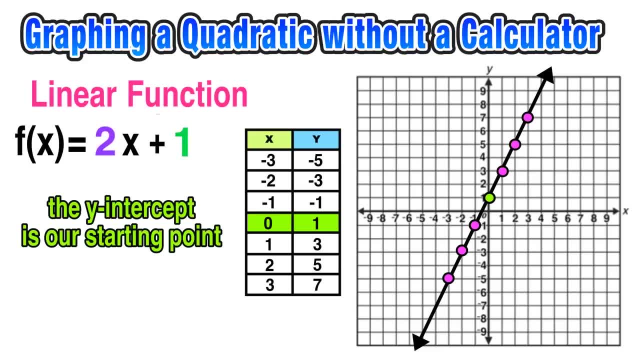 and we use the slope to build the line, fill in a table and construct the graph. So now we want to extend our understanding of graphing linear functions and develop a strategy for graphing quadratic functions which are of the form ax squared plus bx. 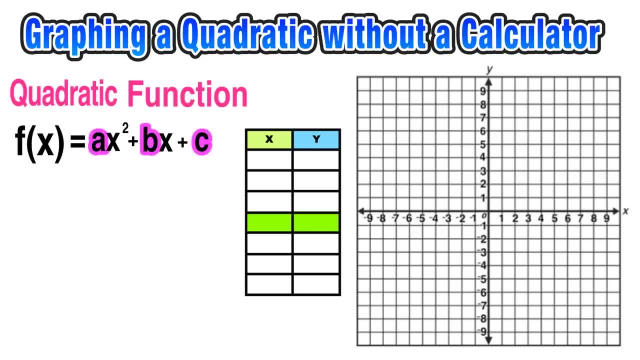 So, for example, let's replace a, b and c- those coefficients, with 1, negative 4 and 5. And also notice that a is 1, so we're just going to drop it, we're not going to include it, So our actual 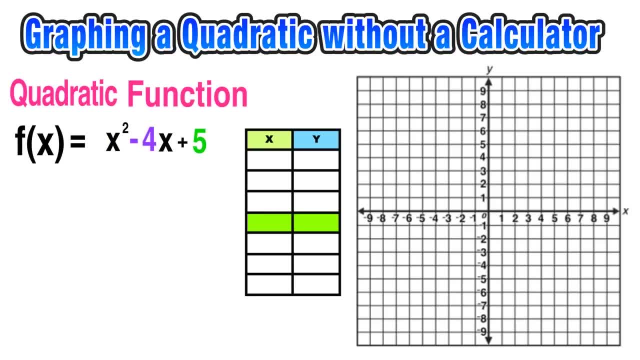 function here is: f of x equals x squared minus 4x plus 5.. That's what we want to graph, And we should also be familiar with the fact that a quadratic function has this curve, this u-shaped graph called a quadratic function. So we're going to be familiar with the fact that a quadratic 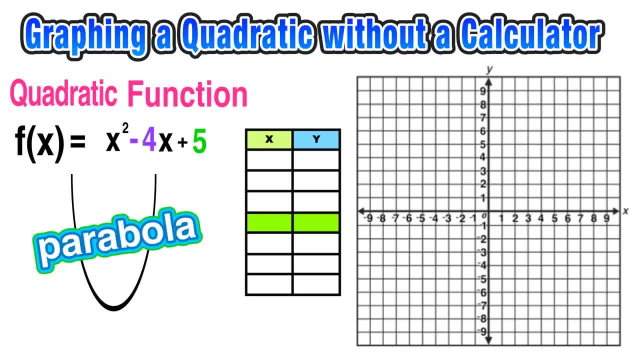 function has this curve, this u-shaped graph called a parabola. Now, with a linear function, the y intercept was the really important point that we could build off of. but with a quadratic function, that important point is that vertex, that turning point, And if we can find that point we can graph. 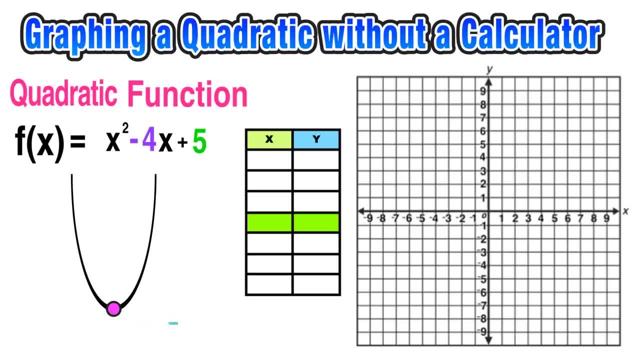 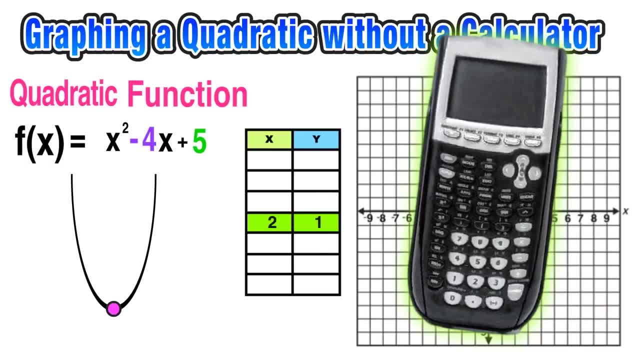 the parabola. Now for quick reference here. you could take that function and put it into y equals on your graphing calculator, and then the calculator would do all the thinking for you. It would fill on the table of values, which would be y equals x squared plus bx squared plus bx squared plus bx squared. 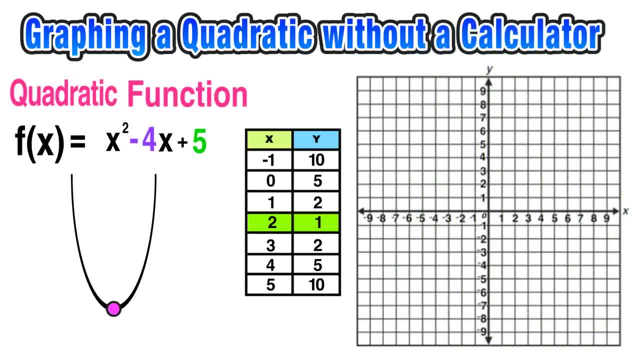 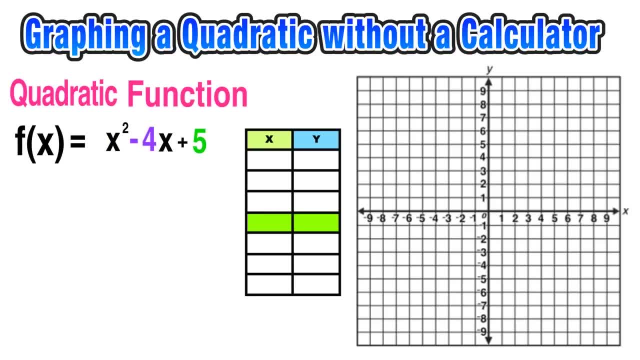 function here is: f of x equals x squared minus 4x plus 5.. That's what we want to graph, And we should also be familiar with the fact that a quadratic function has this curve, this u-shaped graph called a quadratic function. So we're going to take a quadratic function and we're going to 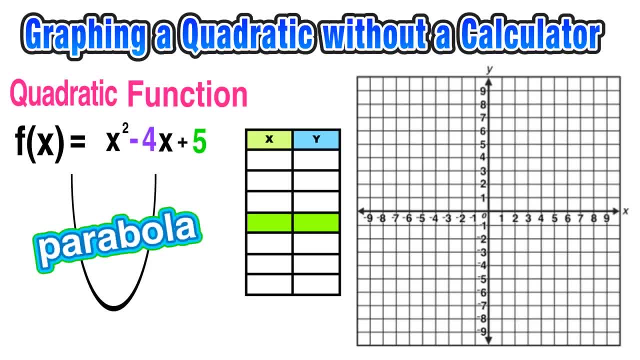 call it a parabola Now. with a linear function, the y-intercept was the really important point that we could build off of. But with a quadratic function, that important point is that vertex, that turning point, And if we can find that point we can graph the parabola. Now for quick. 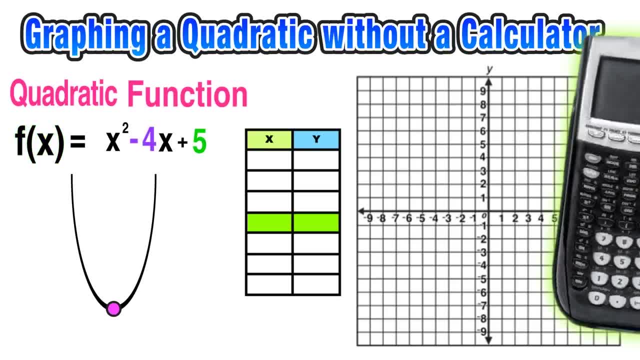 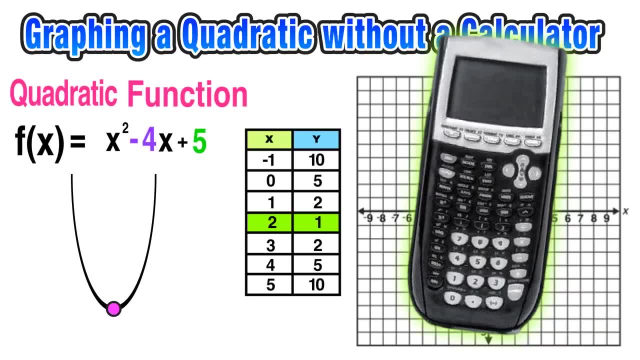 reference here. you could take that function and put it into y equals on your graphing calculator, And then the calculator would do all the thinking for you. It would fill in the table of values, and all that you would have to do with that table of values is plot the. 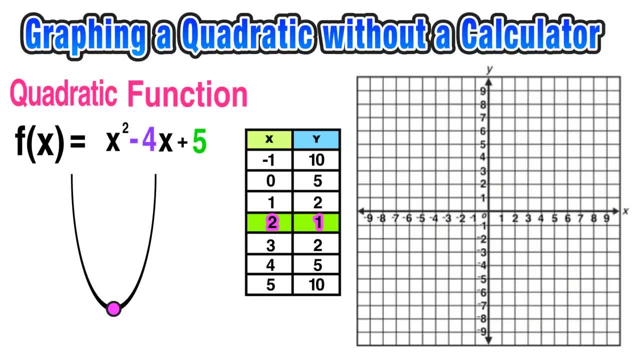 point, starting with the vertex, in this case at, and then again, provided that you have that table of values, you can go ahead and plot the rest of the points around the vertex, which will allow you to graph the parabola. So we can say that if we know the vertex, then 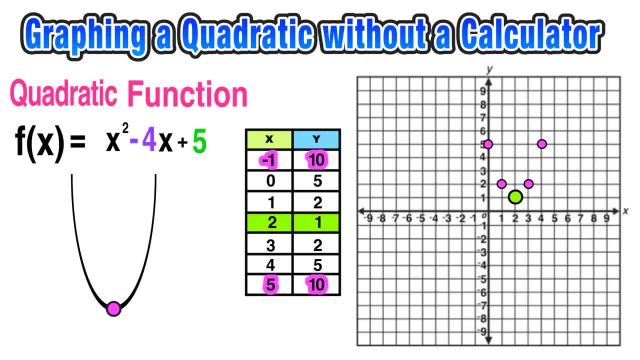 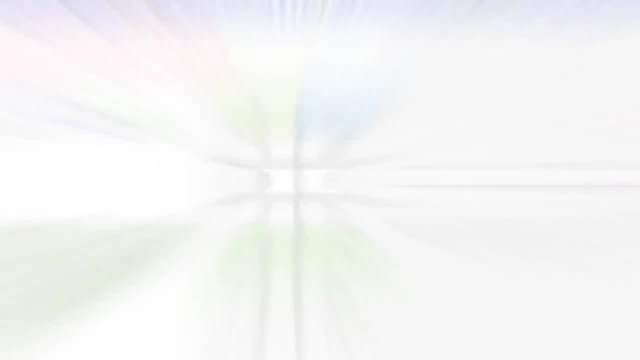 the points around the vertex which will allow you to graph the parabola. So we can say that if we know the vertex, then we can build the parabola and graph the quadratic function. So now let's roll the quadratic function. So now let's take this a step further and explore how we can graph a. 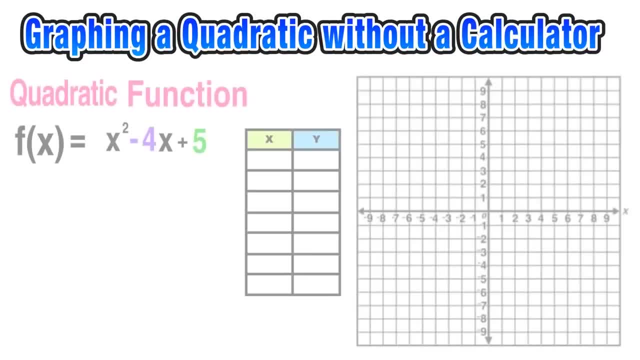 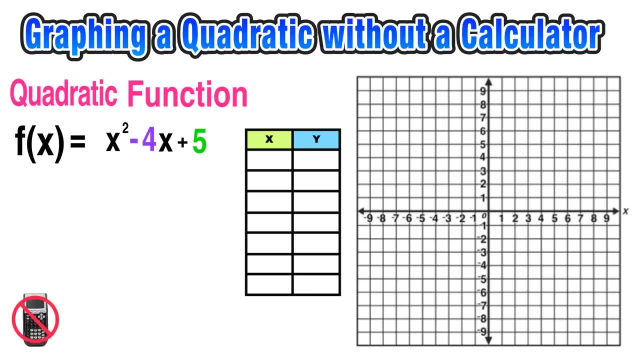 quadratic without using a calculator. So let's go ahead and revisit the last example of f of x equals x squared minus 4x plus 5.. That's the function that we want to graph. In order to do that, we need a table of values. So first thing we want to do is find the vertex of this function. 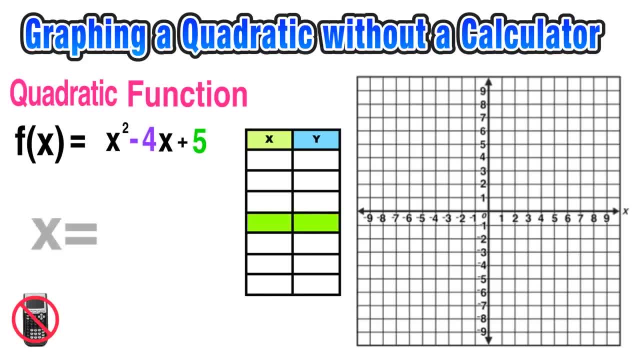 So how do we find it? There is a formula which you may or may not be familiar with: x equals negative b over 2a, and this is the formula for finding the axis of symmetry of a parabola. So let's explore what this means. First, let's replace b in the formula with the b. 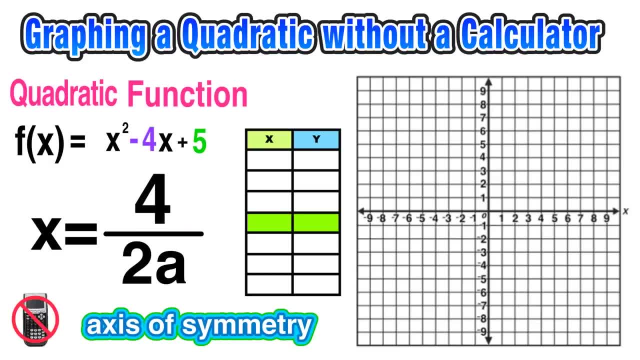 term from the quadratic of negative 4, and then negative negative 4 is just positive 4.. And then down in the denominator 2 times a. We know that the a term is 1, so we're going to get the subway. So let's add in the denominator 2 times a. 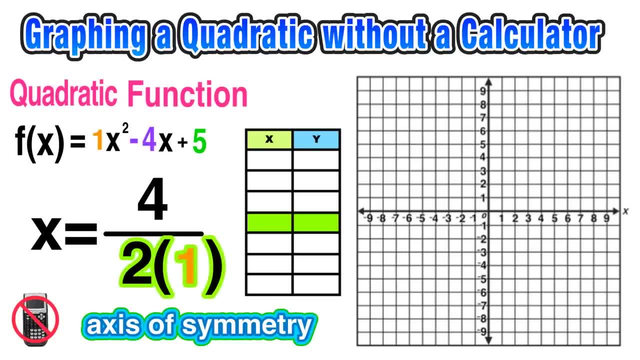 So we're going to add in the denominator 2 times a. So we're going to add in the denominator 2 times a. replace a with 1, and 2 times 1 is just 2.. Finally, we have 4 over 2, or 4 divided by 2, which is just. 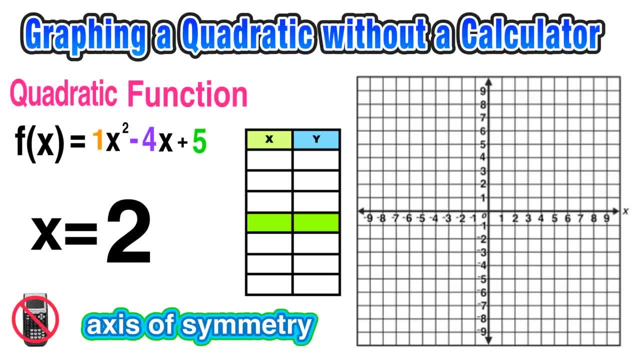 2. So our axis of symmetry is at x equals 2.. Now we know that an x equals equation is a vertical line equation, in this case at positive 2.. Now, what an axis of symmetry is. okay, that is the line that goes through the vertex of the parabola. Now we don't know where that parabola is on the y, but we 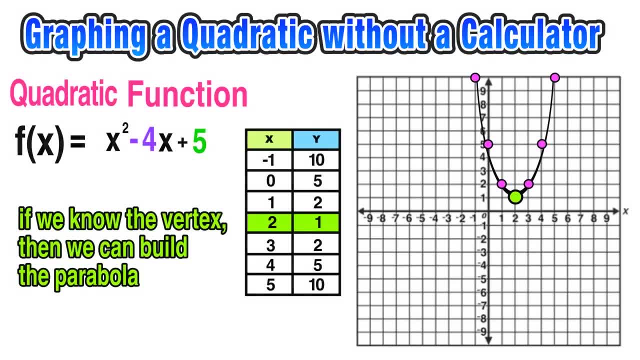 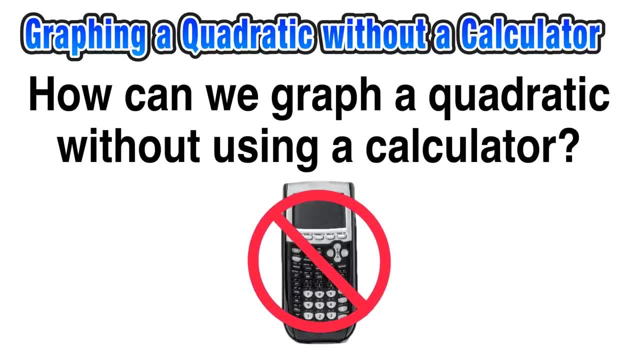 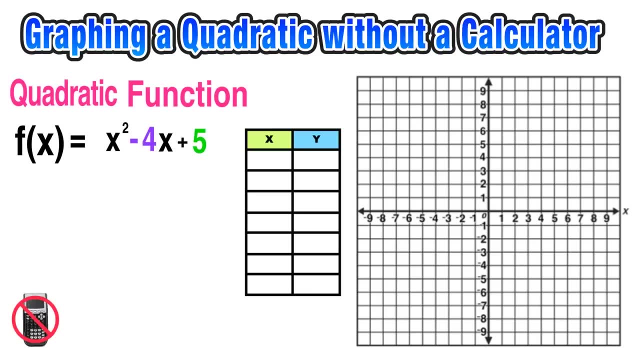 we can build the parabola and graph the quadratic function. So now let's take this a step further and explore how we can graph a quadratic without using a calculator. So let's go ahead and revisit the last example of f of x equals x squared minus four, x plus five. 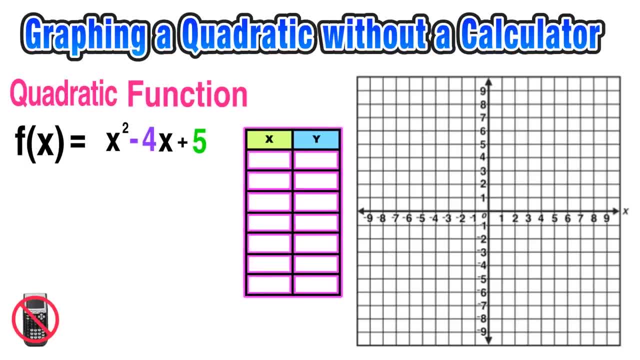 That's the function that we want to graph. In order to do that, we need a table of values, So first thing we want to do is find the vertex of this function. So how do we find it? There is a formula which you may or may not be familiar with: X equals negative b over. 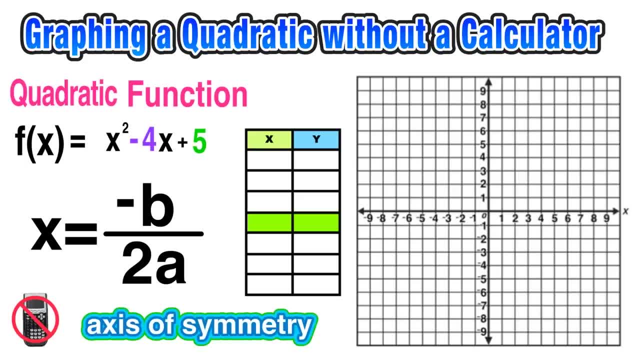 two, a, And this is the formula for finding the axis of symmetry of a parabola. So let's explore what this means. First let's replace b in the formula with the b term from the quadratic of negative four, and then negative negative four is just positive four, And then 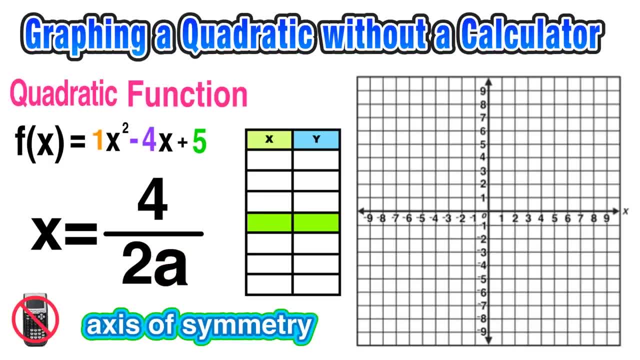 down in the denominator two times a. we know that the a term is one, so I replace a with one And two. 2 times 1 is just 2.. Finally, we have 4 over 2 or 4 divided by 2, which is just 2.. So our 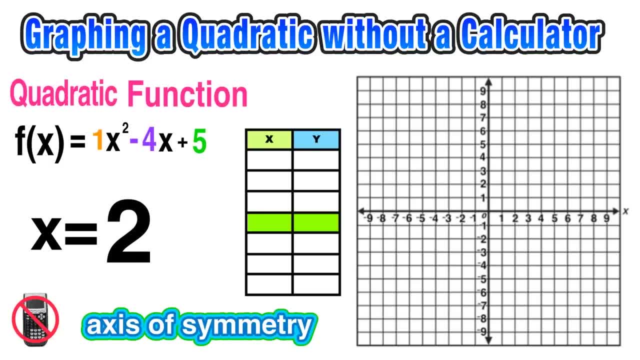 axis of symmetry is at x equals 2.. Now we know that an x equals equation is a vertical line equation, in this case at positive 2.. Now, what an axis of symmetry is. okay, that is the line that goes through the vertex of the parabola. Now we don't know where that. 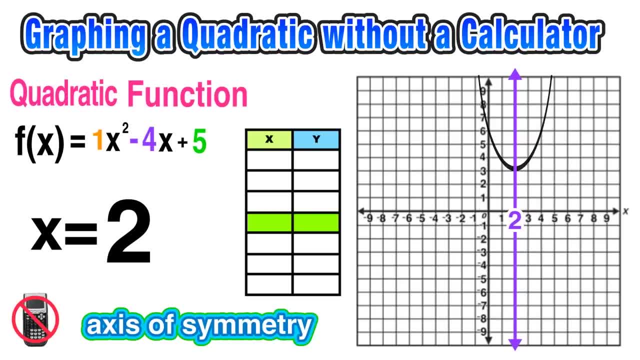 parabola is on the y, but we do know where it is on the x, And that is at positive 2.. So we have the x coordinate of our vertex. Now all we need to do is find the y coordinate, and that is still unknown. However, we do know that x is 2, we just figured that out, And 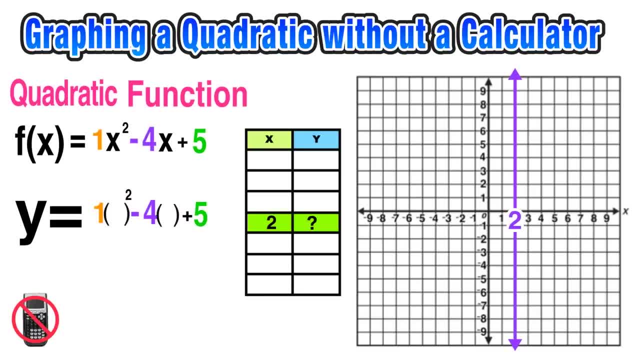 y equals the original quadratic. So I'm going to replace x with 2 and then evaluate. So 1 times 2 squared is 4.. Minus 4 times 2 is negative 8.. And then I just bring down that positive 5.. And 4 minus 8 plus 5 evaluates to just 1.. 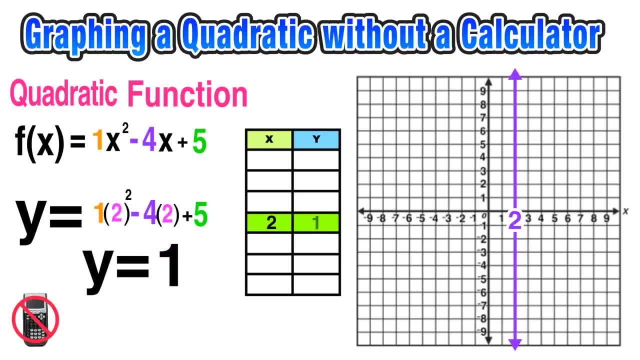 So the y coordinate when x is 2 is positive 1.. And now we have the coordinates of our vertex at 2, 1.. And we can go ahead and plot that point. So to quickly recap what we just did, We found the vertex of this parabola by first using the axis of symmetry formula. 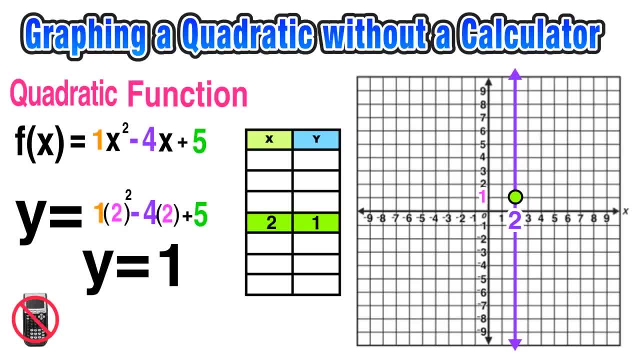 x equals negative b over 2a. Then we plug that x value into the original function to get the output which was the y value of the vertex, And then we had our full point. So now we know that our parabola has a vertex at 2, 1.. And we should have a better idea. 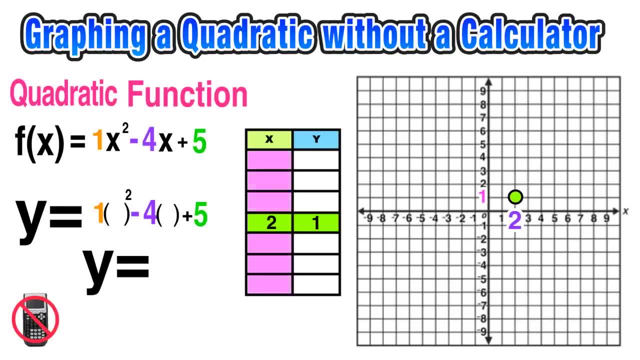 of what our final graph is going to look like, But we still need to find the rest of the points. Now for the x values, I'm just going to build above and below the vertex value. So now, for instance, if I want to find the y value when x is 3.. 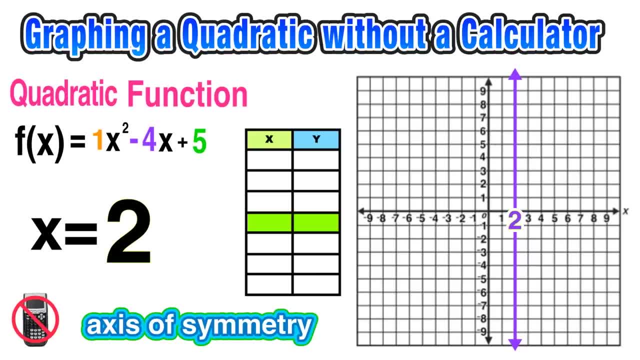 do know where it is on the x, and that is at positive 2.. So we have the x coordinate of our vertex. Now all we need to do is find the y coordinate, and that is still unknown. However, we do know that x is 2- we just figured that out- and y equals the original quadratic. So I'm going to 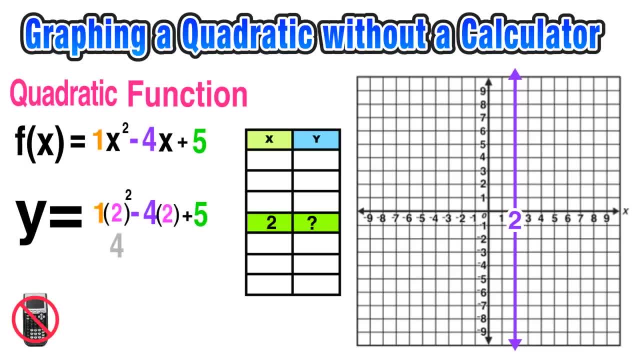 replace x with 2 and then evaluate. So 1 times 2 is 2.. 2 times 2 squared is 4.. Minus 4 times 2 is negative 8.. And then I just bring down that positive 5. And 4 minus 8 plus 5 evaluates to just 1.. So the y coordinate when x is 2: 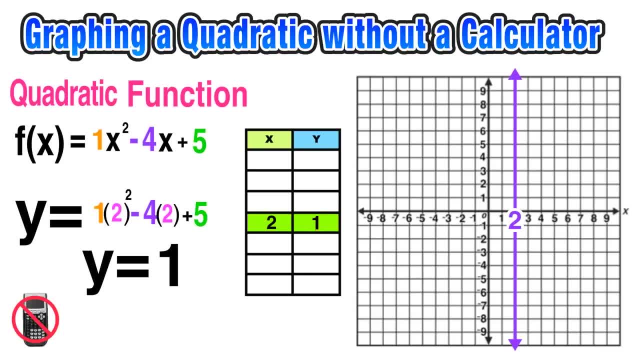 is positive 1.. And now we have the coordinates of our vertex at 2, 1.. And we can go ahead and plot that point. So to quickly recap what we just did, we found the vertex of this parabola by first using 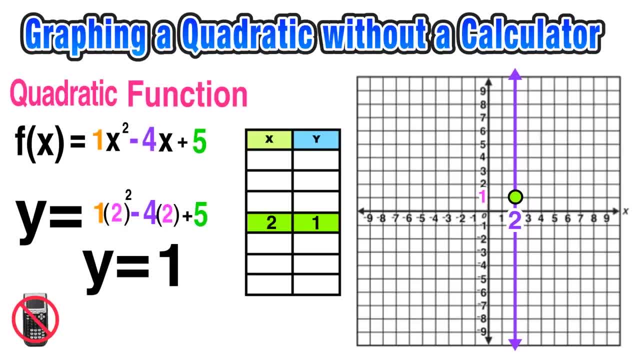 the axis of symmetry And then we can go ahead and plot that point. So to quickly recap what we just tried, we have the axis of symmetry, formula x equals negative b over 2a To find the x value of the vertex. Then we plug that x value into the original function to get the output which was the. 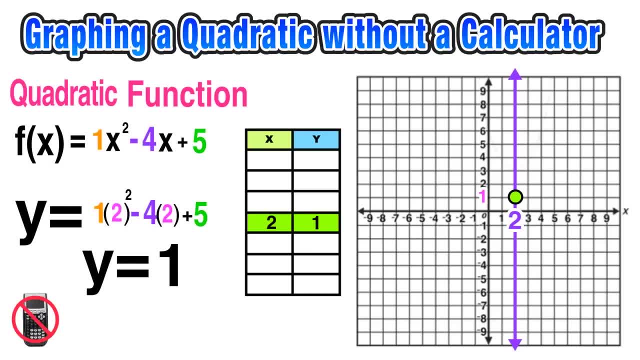 y value of the vertex, and then we have our full point. So now we know that our parabola has a vertex at 2, 1.. And we should have a better idea of what our final graph is going to look like. But 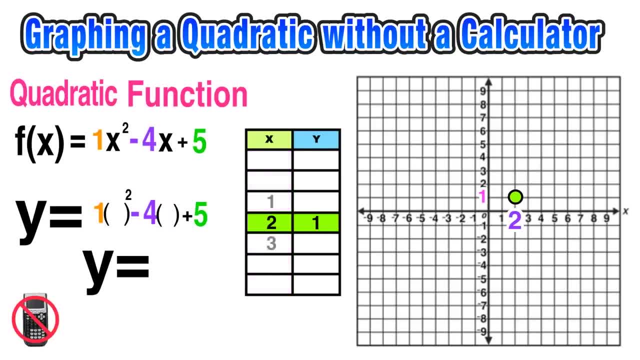 we still need to find the rest of the points. Now for the x values, I'm just going to build above and below the vertex values. So we're going to use this for our final graph And we're just going to So now. for instance, if I want to find the y value when x is 3, I will replace x in the original function with 3 and then just evaluate. 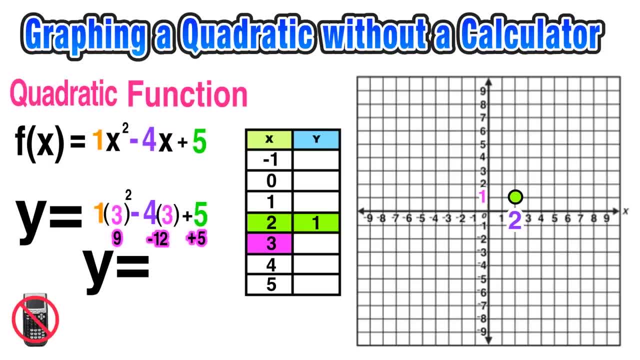 So in this case I would have 9 minus 12 plus 5, which evaluates to positive 2.. So when x is 3, y is positive 2.. And now I have another point on the parabola, So I'm going to go ahead and plot the point 3, 2.. 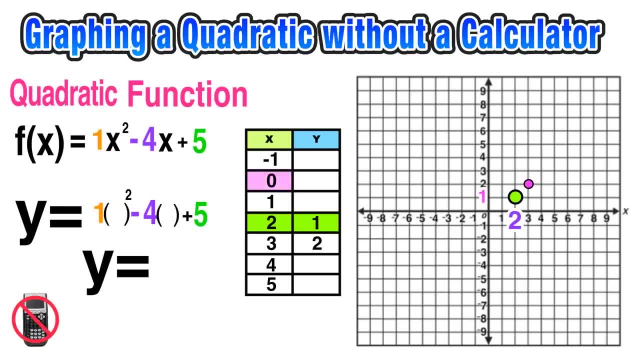 Let's go ahead and find another point. Let's say I want to find the y value when x is 0. I'll replace x with 0 in the original function and then evaluate And I should just get positive 5.. So 0, positive 5 is another point. that is on the parabola. 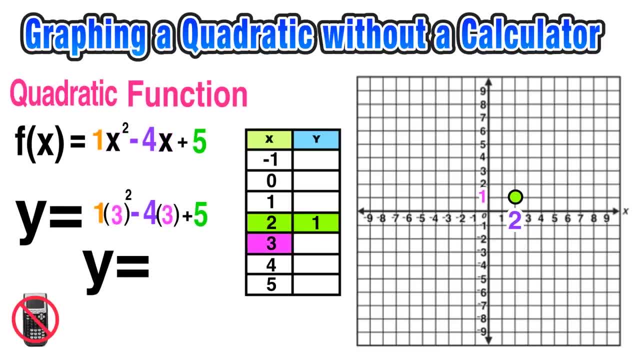 I will replace x in the original function with 3 and then just evaluate. So in this case I would have 9 minus 12 plus 5, which evaluates to positive 2.. So when x is 3, y is positive 2.. And now I have another point on the parabola, So I'm going to go ahead. 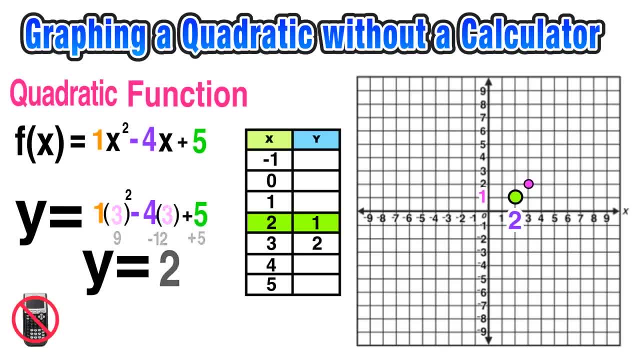 and plot the point. Let's go ahead and find another point. Let's say I want to find the y value when x is 0. I'll replace x with 0 in the original function And then evaluate, And I should just get positive 5.. So 0, positive 5 is another point that is. 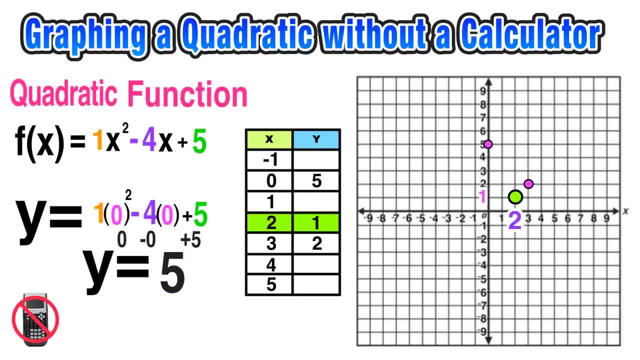 on the parabola, And now I can easily repeat this process for the remaining x values to find the rest of the points that are on the graph. Now, once I do this, I have a filled in table of values And all I have to do is plot those remaining points And we have completed. 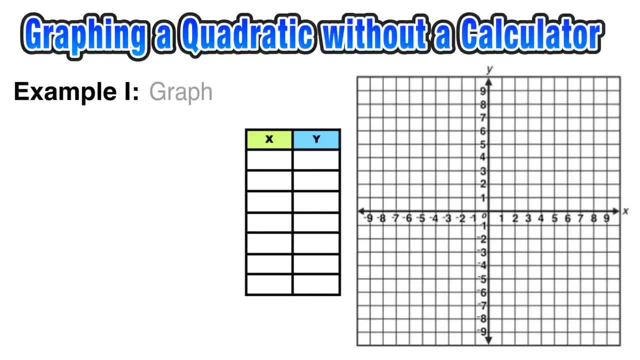 our graph. Haha, cool, Okay. so let's try one more example here. We want to graph the quadratic f of x equals x squared minus 2x minus 6, without using a calculator. Now, remember that the first thing we want to find is the vertex of the parabola, And then we can build from there. Now again, 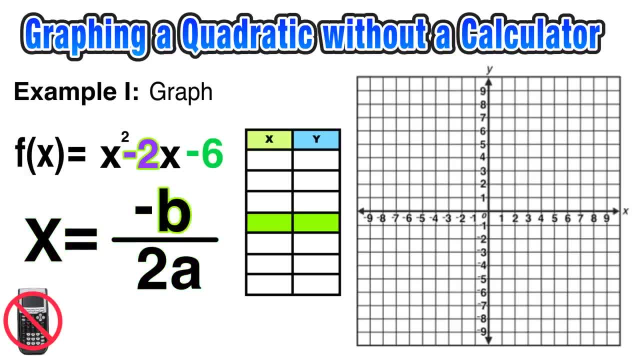 we want to use that axis of symmetry. formula x equals negative b over 2a And we're going to fill in and evaluate, Replace b with negative 2.. Negative negative 2 is just positive 2.. And then in a denominator we replace a with the. 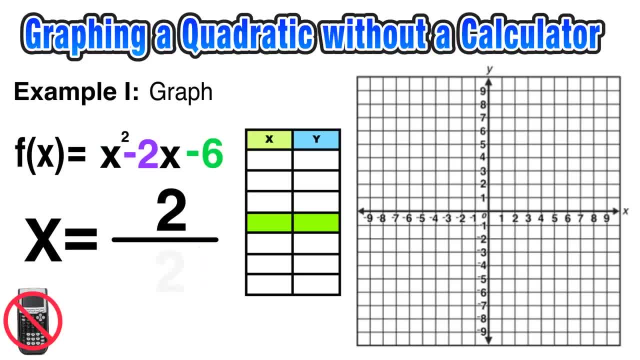 a value, In this case just one, And 2 times 1 is just 2.. Finally,2 over 2, or 2 divided by 2, is just equal to 1.. And now we have the x coordinate for our vertex at positive 1.. So now we're going to use that value of positive 1 to plug in. 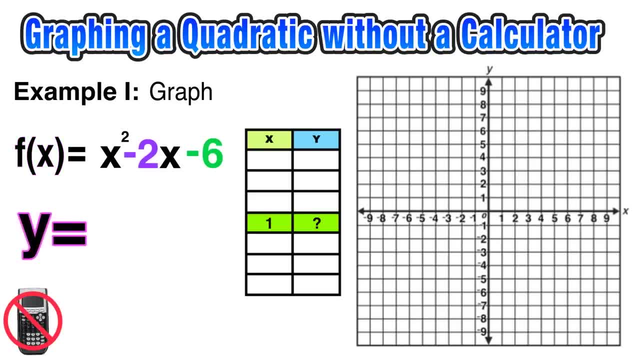 and find the value of y. Now remember that f of x equals and y is equal to 4b, which equals mean the same thing. so I rewrite the function in y equals form and then I replace the X's with 1 and now I can evaluate 1. squared is just 1 negative 2. 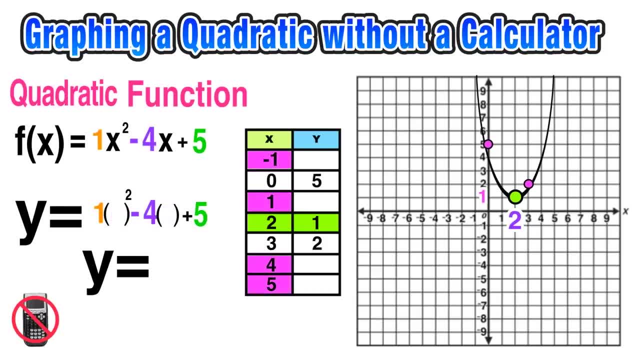 And now I can easily repeat this process for the remaining x values to find the rest of the points that are on the graph. Now, once I do this, I have a filled in table of values And all I have to do is plot those. 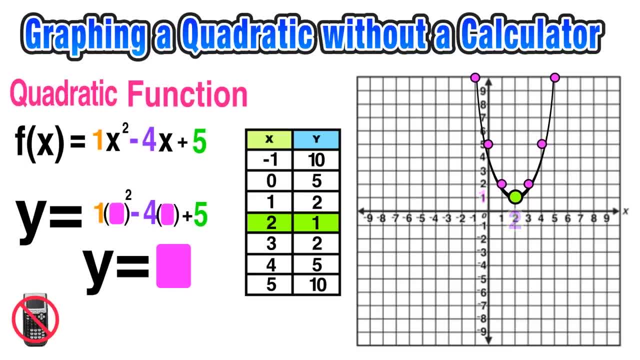 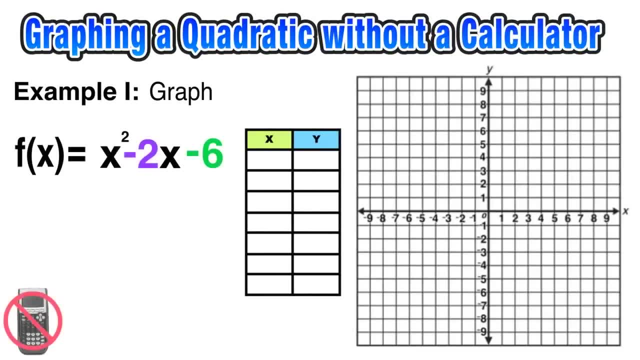 Those remaining points and we have completed our graph. Okay, so let's try one more example here. We want to graph the quadratic f of x equals x squared minus 2x minus 6, without using a calculator. Now, remember that the first thing we want to find is the vertex of the parabola. 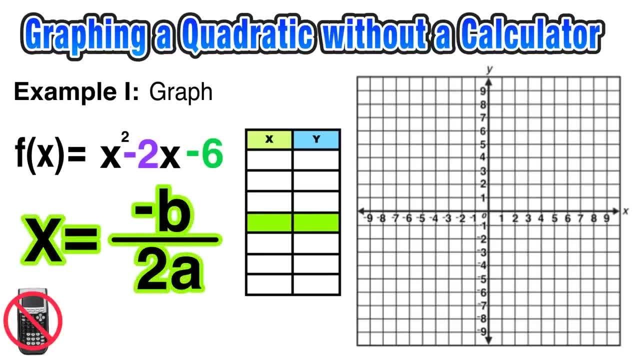 And then we can build from there. Now again, we want to use that axis of symmetry. formula x equals negative b over 2a And we're going to fill in and evaluate. Replace b with negative 2.. Negative, negative 2 is just positive 2.. 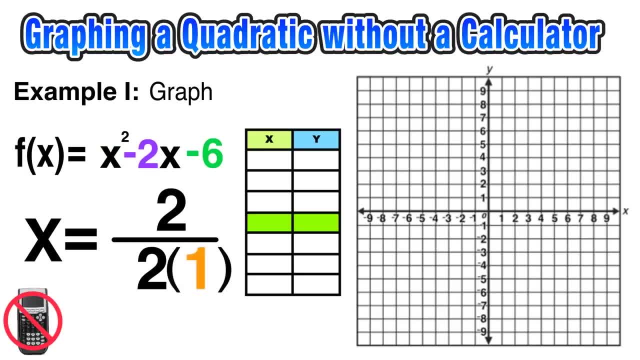 And then in the denominator we replace a with the a value, In this case just 1.. And 2 times 1 is just 2.. Finally, 2 over 2 or 2 divided by 2 is just equal to 1.. 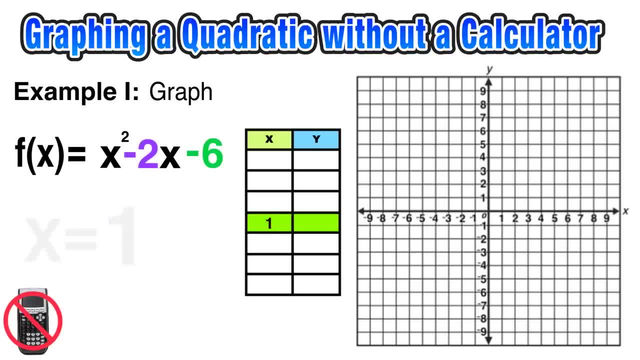 And now we have the x coordinate for our vertex at positive 1.. So now we're going to use that value of positive 1 to plug in and find the value of y. Now remember that f of x equals and y equals mean the same thing. 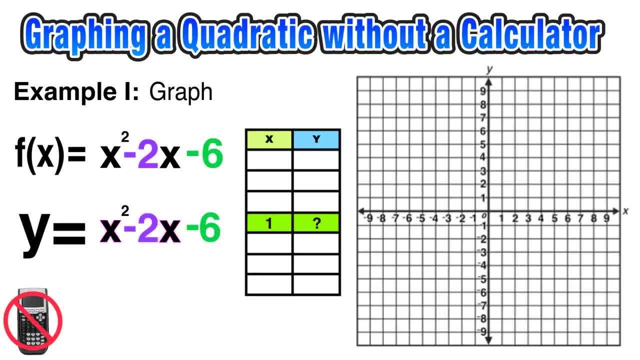 So I rewrite the function in y equals form And then I replace the x's with 1.. And now I can evaluate: 1 squared is just 1.. Negative 2 times 1 is just negative 2.. And then I just bring down that negative 6.. 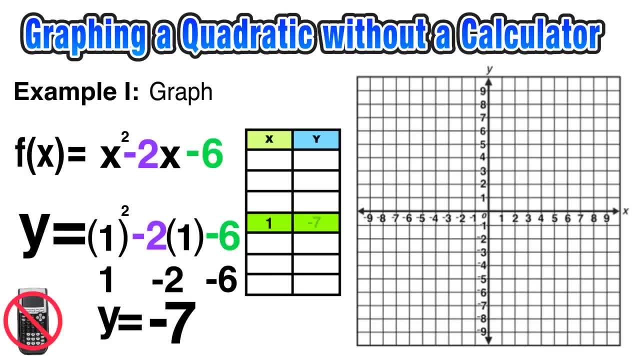 And then 1 minus 2 minus 6 is equal to negative 7.. And that is the value of our y coordinate, of our vertex. So we found the vertex and it is at 1, negative 7.. So I can go ahead and plot that point. 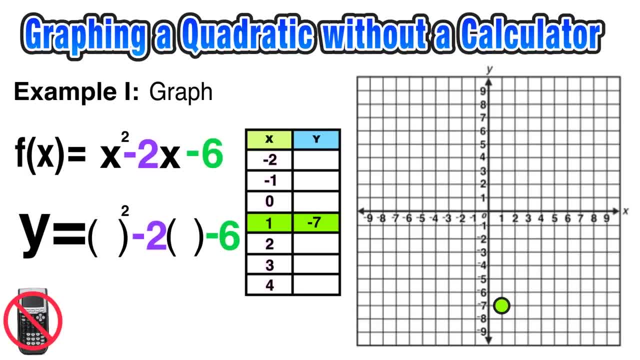 Next I can go ahead and fill in the x values on my table of values by going above and below the x value of the vertex, And now I'm ready to find the rest of the points on the parabola. So if x is negative 2, I replace it in the original function with negative 2 and then evaluate. 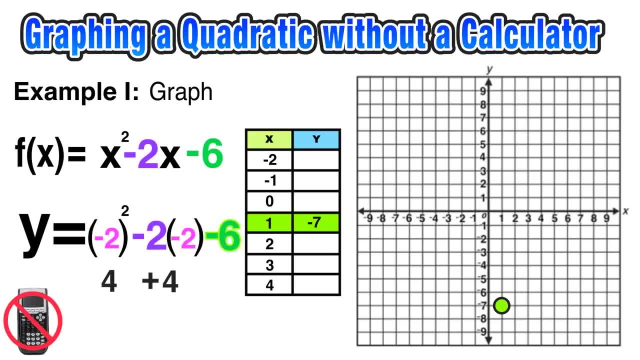 In this case I would have 4 plus 4 minus 6. Which evaluates to positive 2.. So when x is negative, 2,, y is positive 2.. And I have another point: negative 2, 2, that is on the graph. 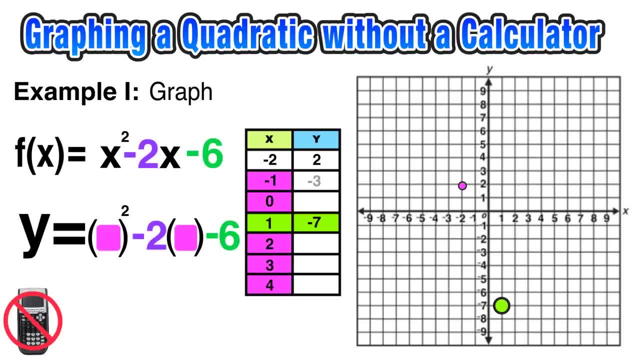 And now all you have to do is repeat this process for the remaining x values by substituting it in, And whatever your output is, that will be your y value. Now, once you have these remaining points and you have completed your table of values, you can plot them on the graph and construct your parabola. 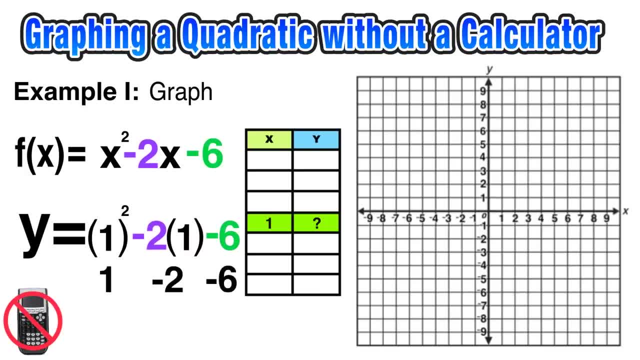 times 1 is just negative 2, and then I just bring down that negative 6, and then 1 minus 2 minus 6 is equal to negative 7, and that is the value of our y coordinate, of our vertex. so we found the vertex and it is at 1 negative 7. so I 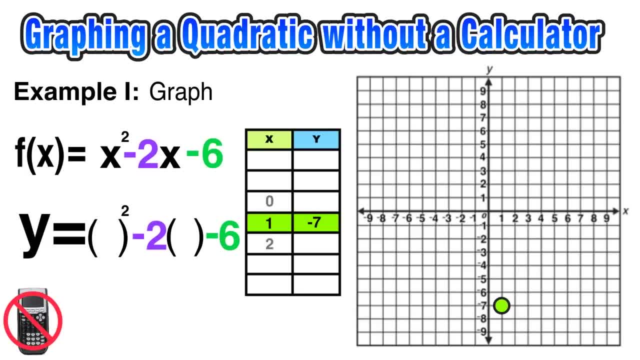 can go ahead and plot that point. next, I can go ahead and fill in the X values on my table of values by going above and below the X value of the vertex, and now I'm ready to find the rest of the points on the parabola. so if X is negative, 2 I 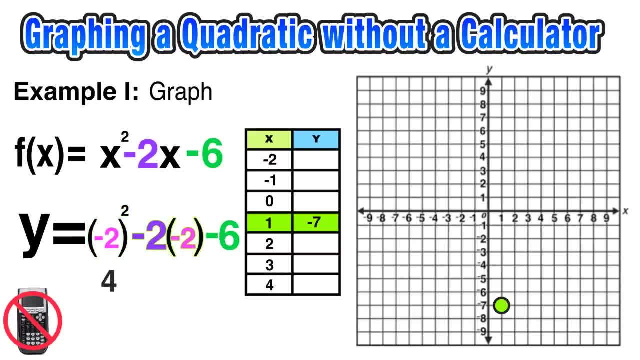 replace it in the original function with negative 2 and then evaluate. in this case I would have 4 plus 4, and then I would have 4 plus 4, and then I would have 4 plus 4, and then I would have 4 minus 6, which evaluates to positive 2. so when X is negative 2, Y is positive 2. 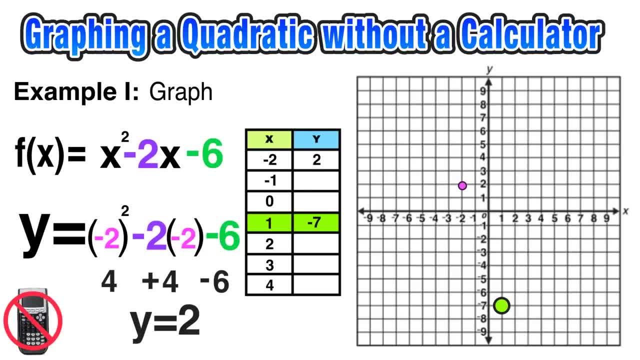 and I have another point: negative 2, 2. that is on the graph, and now all you have to do is repeat this process for the remaining X values by substituting it in, and whatever your output is, that will be your Y value. now, once you have, 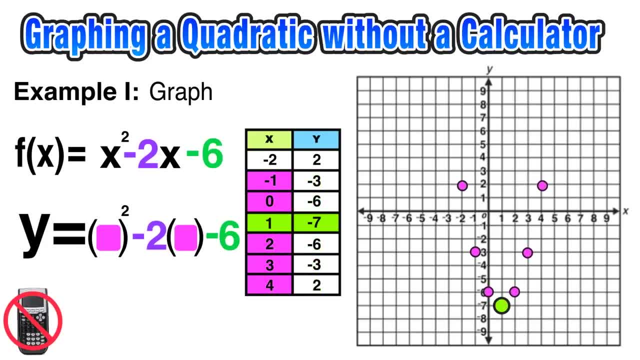 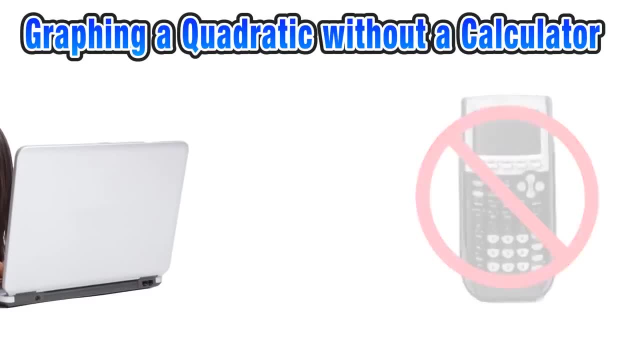 these remaining points and you have completed your table of values. you can plot them on the graph and construct your parabola. and that is how you graph a quadratic function without using a calculator. quick recap: whenever you want to graph a quadratic function without the use of the calculator, you start by: 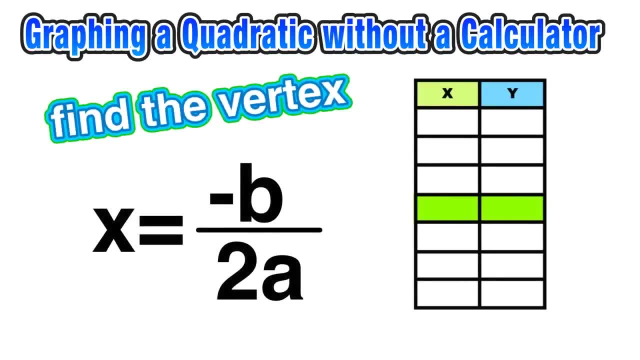 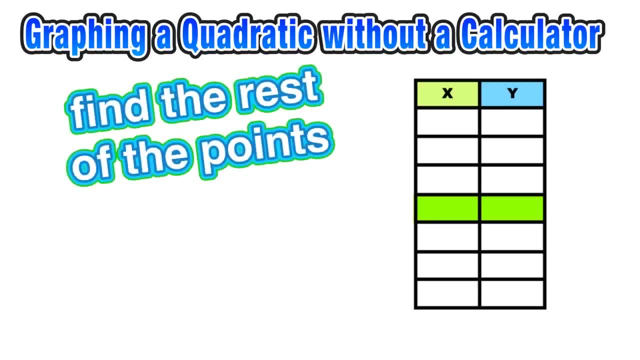 finding the vertex point using the X equals negative B over 2a formula. once you find X, you plug it into the original function to get your value of Y. then you find the rest of the points by plugging the X values into the original function, then plotting your points in your table of values. 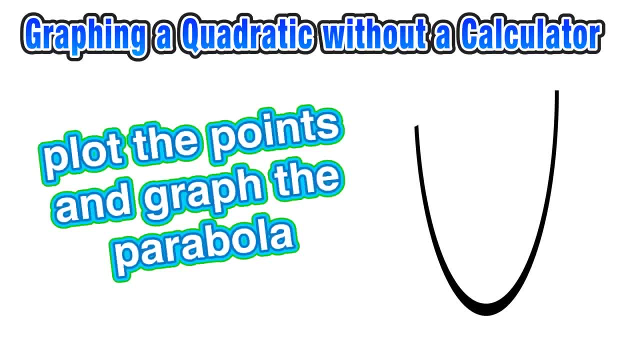 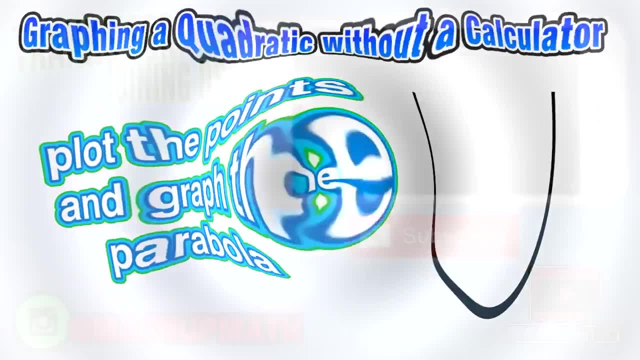 and constructing your graph. that's all there is to it. so practice this, think about what you're doing so you understand the concept in addition to the procedure, and we'll catch you guys next time. thanks again, guys. I'm glad that you like our video lessons. if you don't know, we have an awesome, awesome. 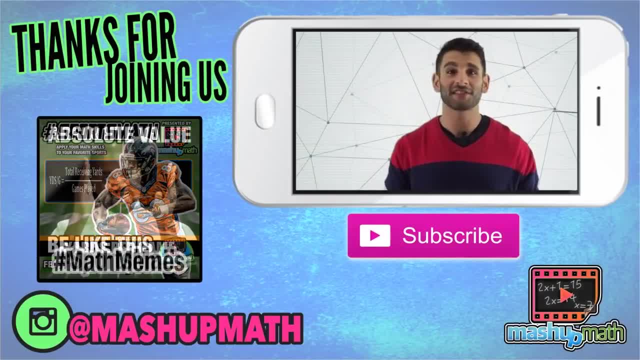 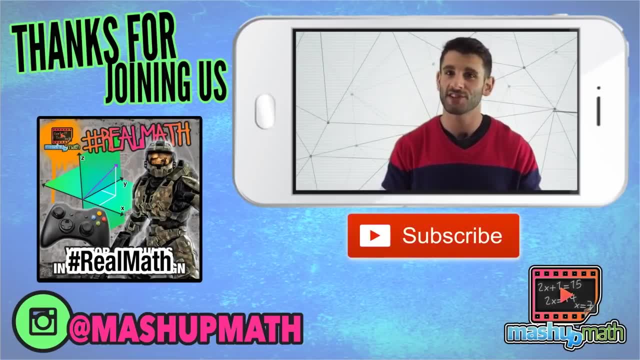 really awesome Instagram page at mashup math. that's the first thing we ever started with, so we have some really cool sports math posts. we do daily math tips, all kinds of study tips, tips for parents, tips for teachers- you're really gonna like it. very artistic, very colorful, very.